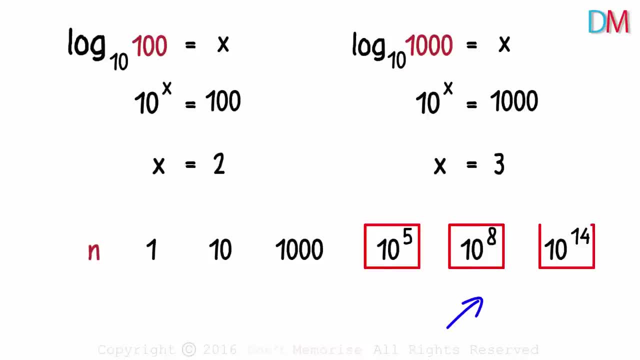 This is the approximate distance from the earth to the sun And this is the approximate number of cells in the human body. Now assume you have been asked to plot the following values on a number line. How would you do it? We cannot mark natural numbers like this, because these large numbers won't really fit into. 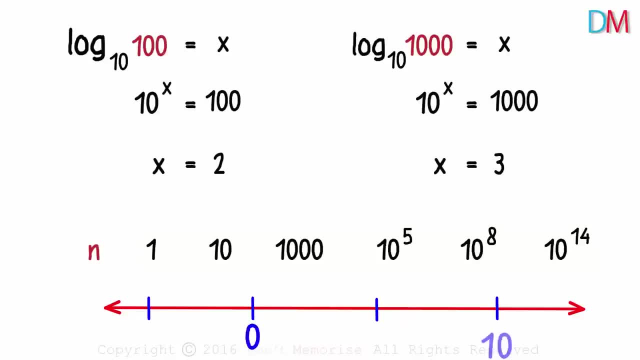 our little notebooks. If we mark 0 and 10 raised to 14 here, these tiny numbers like 1, 10 and 1000 would be super close to 0. So what's the solution? How about we take the logarithm of the numbers to the base 10?? 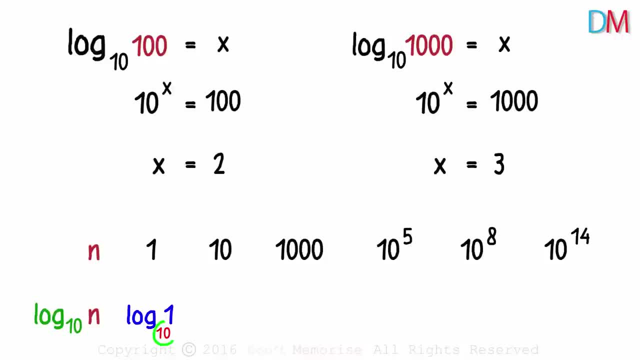 What will be the log of 1 to the base 10?? 10 raised to 0 is equal to 1.. Hence we have a 0 here. Log 10 to the base 10 will equal 1, as 10 to the power 1 will give us 10.. 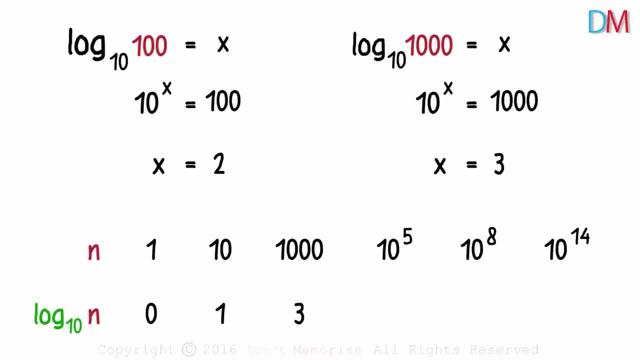 Log of 1000 to the base 10 will equal 3, as 10 cubed is 1000.. Similarly, We get 5, 8 and 14 here. Now I want you to tell me: can these numbers be easily plotted on a number line? 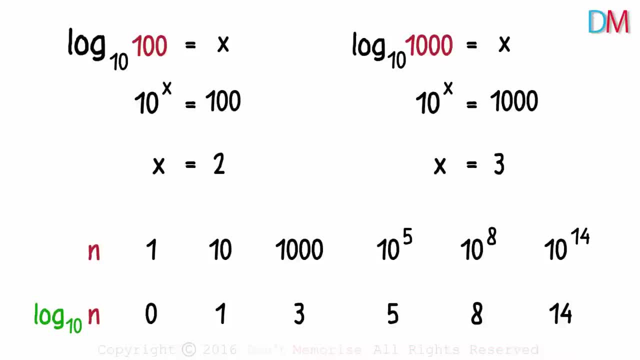 Yes, A scale from 0 to 14 is enough. Large numbers can be easily plotted using logarithms. Also, notice that there is a very large variation between numbers. Logs also help us in narrowing down these variations. So in layman terms we can say that if the events vary drastically, 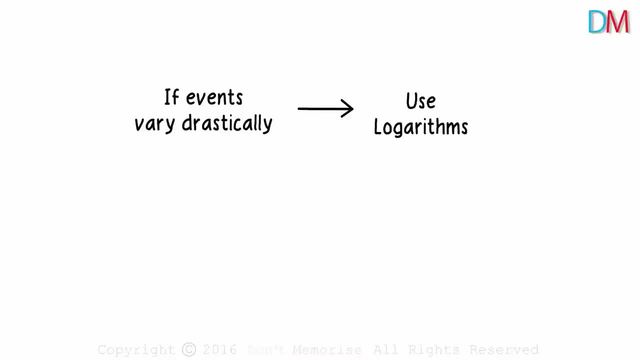 Logs also help us in narrowing down these variations. Logs also help us in narrowing down these variations. As students these days we can use logarithms, And a very common example of that is the Richter scale, which is used to measure earthquakes. It uses a logarithmic scale. 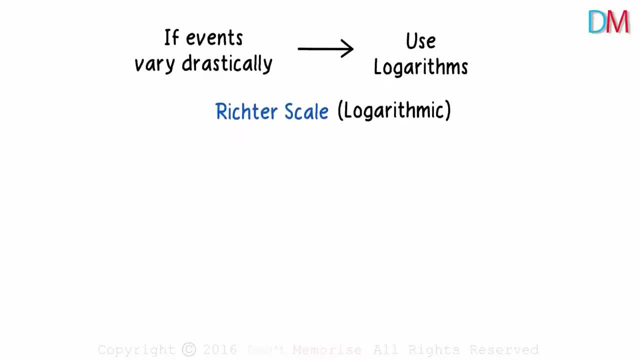 To understand this, let's talk about the earthquakes that happened in three different countries. In India, there was an earthquake that registered a 6.0 on the Richter scale. In the US, there was an earthquake that registered 7.0. and Japan had an earthquake that registered 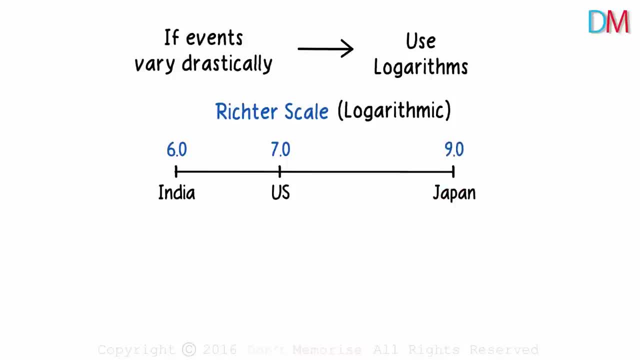 a 9.0 on the Richter scale. But where are the earthquakes? Let's talk about that Now. what does this really tell us? The Richter scale is a base 10 logarithmic scale, Which means they are in the form log M to the base 10..